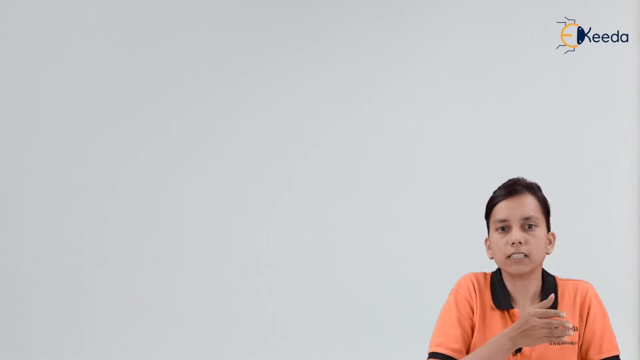 actually transmitting the bit, it is rotating the bit. then I will say that this particular circuit is a shift register For many arithmetic operations. we need this kind of operation that I want to rotate my bit At that time. we require to design such a circuit which has a operation which can: 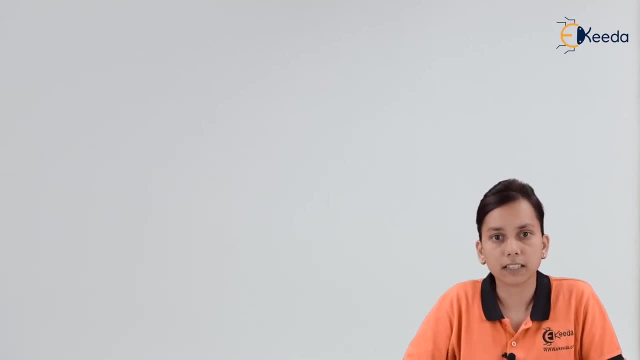 actually perform operation of shifting and that circuit is nothing but our shift register. So basically, shift register can shift in a left manner or a right manner. in this way I can also define the types of the shift register. if it is shifting in a right direction, then I will call. 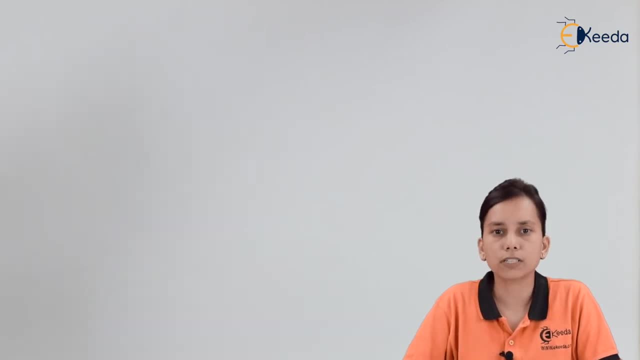 that particular shift register as a right shift register. if it is transferring or rotating the bit in a left direction, then I will call that particular register shift register as shift register, left register. it is up to our requirement that what kind of circuit we want to design. and one more point which is always need to understand is that 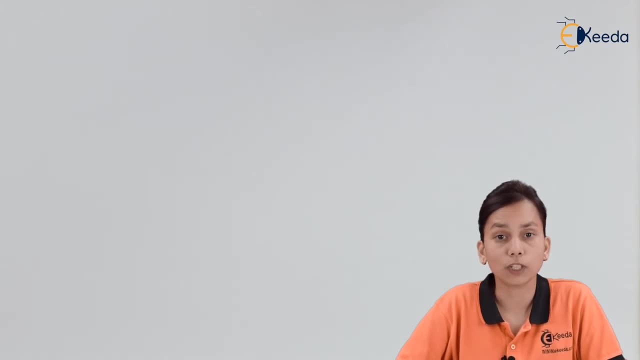 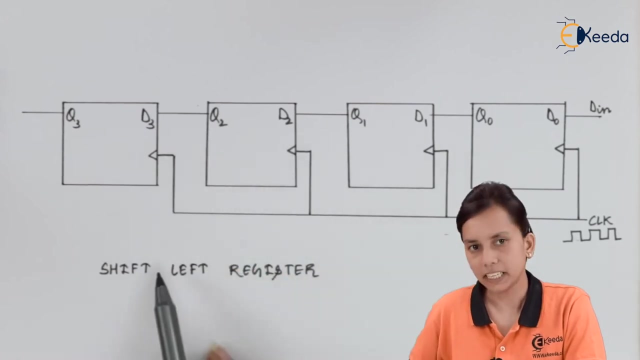 flip-flop is nothing but the basic element of the register. so let us try to understand the working, how we can define, how we can design and how we can get our required output with the help of this shifter register. we will use the D flip-flop to understand the shifter register, as you, we can see on the screen. 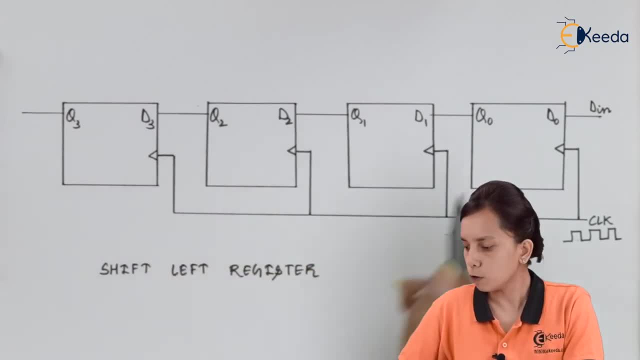 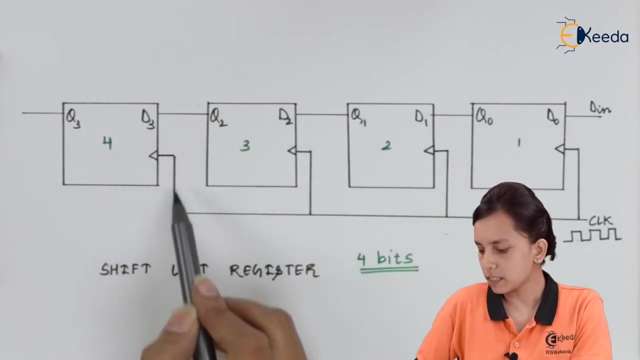 this is the shifter register, which consists of four flip-flops: one, two, three and four. so by this four flip-flop, we can easily understand that it will hold up to four flip-flops, four bits. now it consists of D flip-flop and the clock pulses. these are: 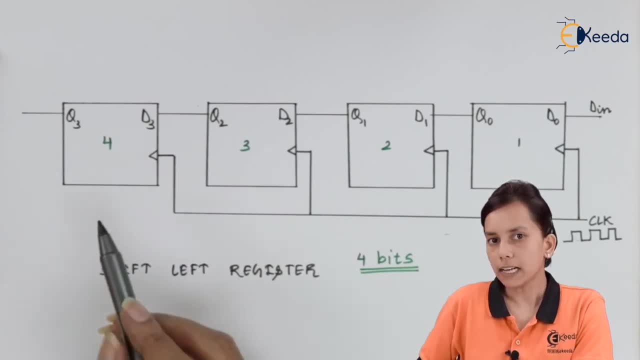 common for all the flip-flops, as we are applying D input here at the one, and let me say that D input is one, as we know that the basic curve operation of the D flip-flop is that if we are applying input, D is equals to one. our output is 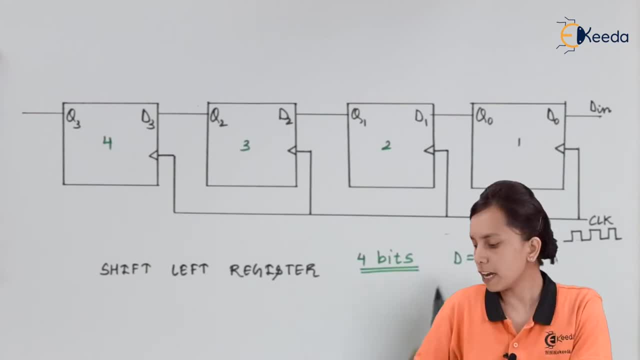 also equals to one one. if we are applying D is equals to zero or output is will be equals to zero. this is very important that whenever we are designing any kind of circuit and whatever flip flop we are using, so first of all we will understand that how the 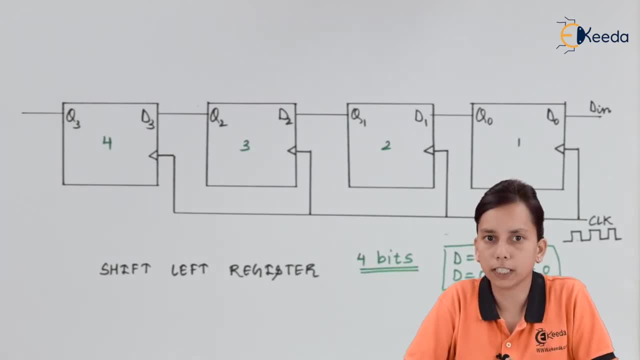 particular type of flip-flop is working. if it is a D flip flop, then if D is equals to one, equals to 1.. My output is also equals to 1.. If I am applying the clock pulse and D is equals to 1, then I will say that output is also equals to 1.. Again, I will apply a clock pulse. Now D is equals. 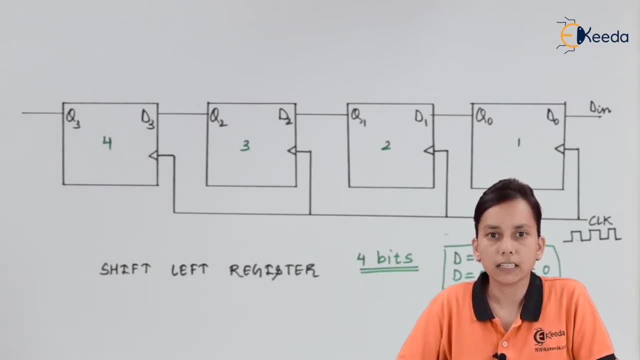 to 0.. My output will also be equals to 0.. Let us understand that, why I am saying that this particular register is a shift register and how we can say that it is shifting in a right direction or in a left direction. Let us say we are applying D- input is equals to 1 and we are applying our. 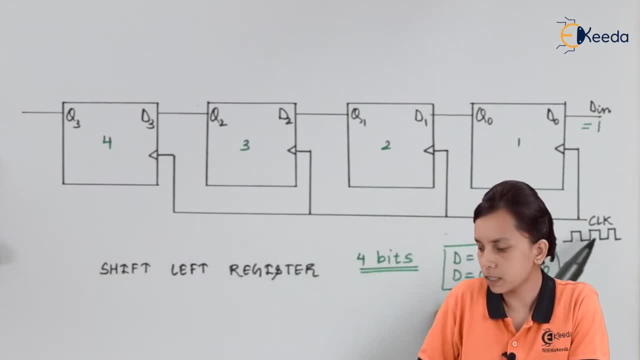 first, clock pulse. This is our clock pulse and we are using positive clock pulse. It means that whenever it is at a 1 stage, whenever clock pulse is at a high stage, I will get output. Now D input is equals to 0.. 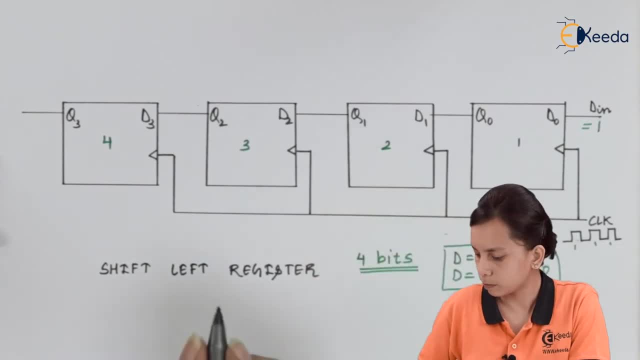 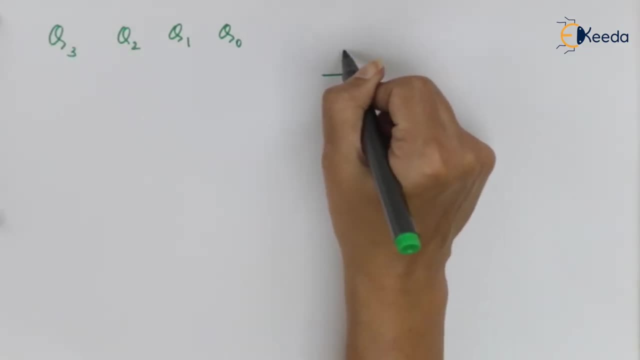 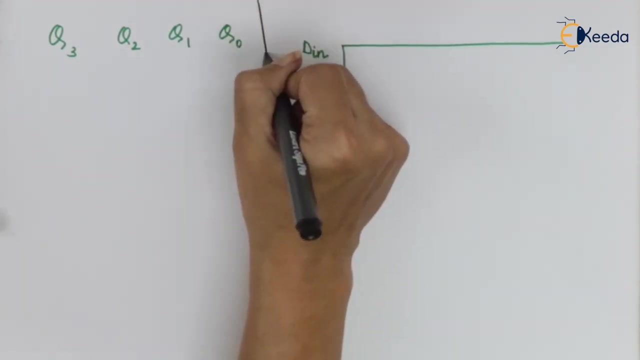 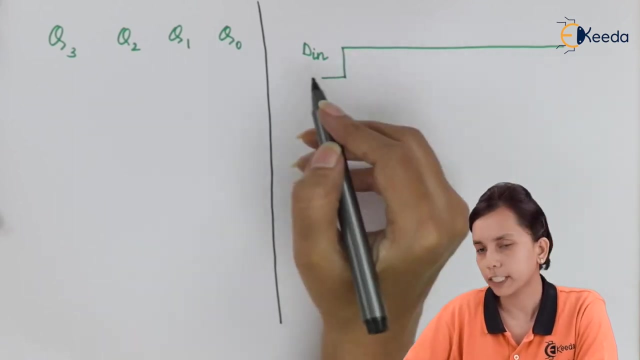 If D input is equals to 1, Q0 will be equals to 1.. Let me write down it here. Let us say, when I am saying that D input is 1. It is constantly equals to 1 and I am applying the clock pulse First clock pulse. 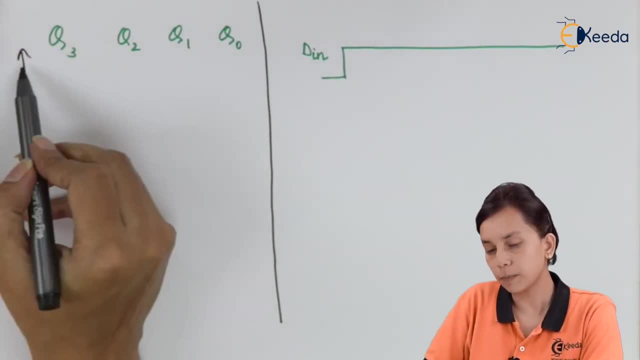 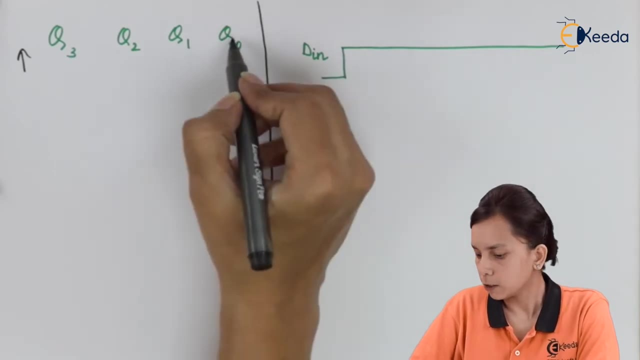 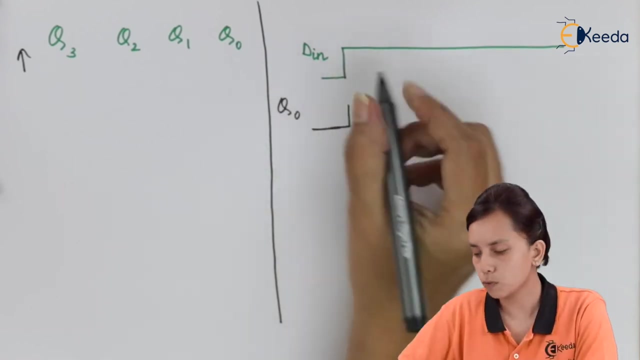 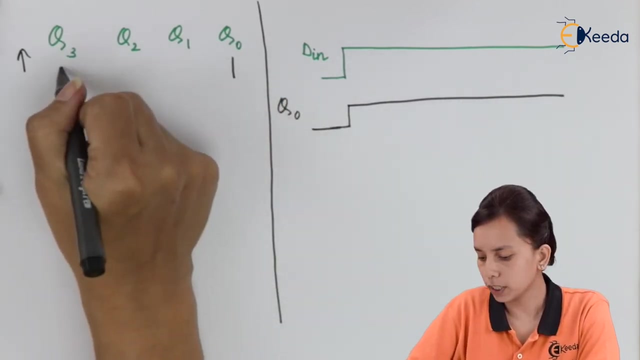 Let us say: the meaning of this arrow is that upward arrow, that I am applying a clock pulse. Now, when I am applying a clock pulse, Q0 will be equals to. if D input is 1, Q0 will always be equals to 1, and Q3,, Q2, Q1 is 0 because they have a clock pulse. 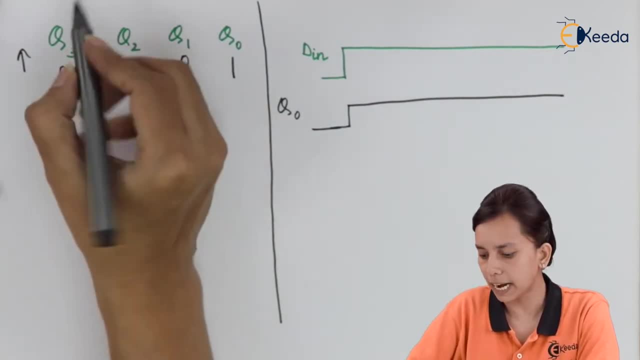 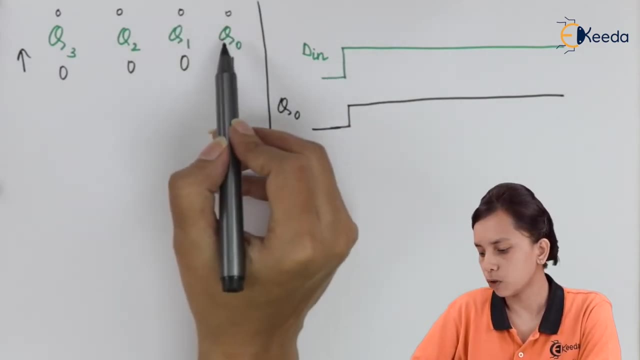 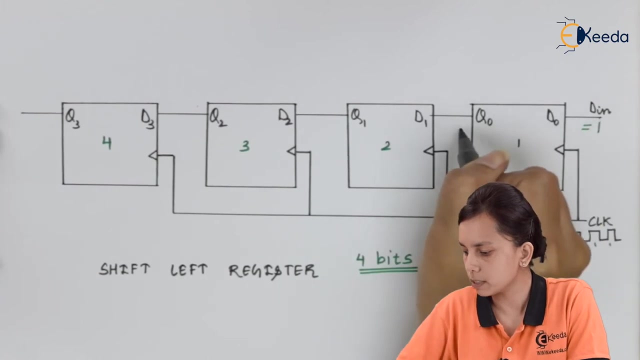 When I am applying, I am applying a first step. There is already a stage, which is assuming that the previous stage was a clear stage. 000.. I applied 1 and Q0 is at 1.. Again, next clock pulse. We applied D input is equals to 1, Q0 is 1 at. 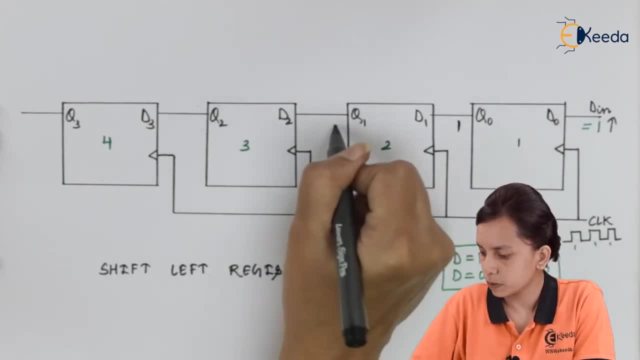 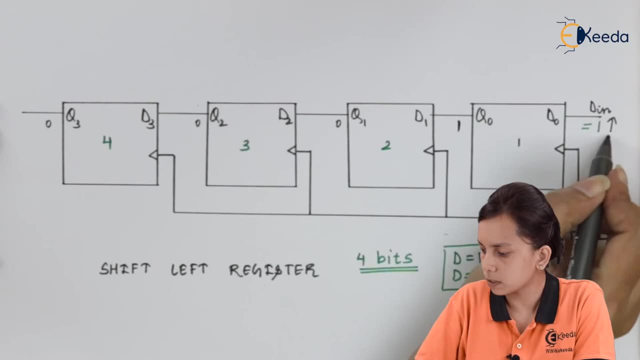 1 at 1.. At first clock pulse This was 0. This is 0.. This is 1.. this is 0.. This is 0.. Now applied second clock pulse: Still, the input is 1.. So this will be equals to 1.. 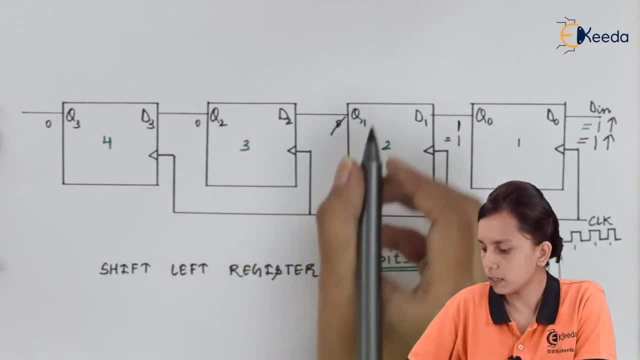 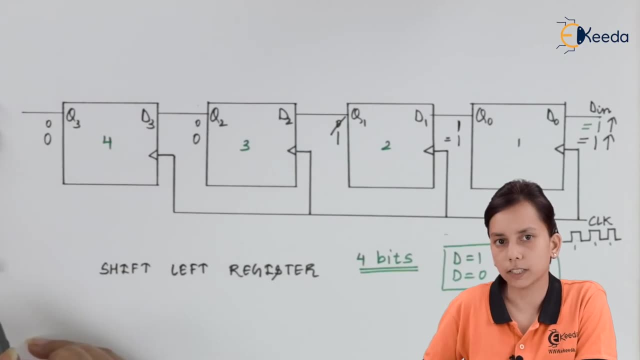 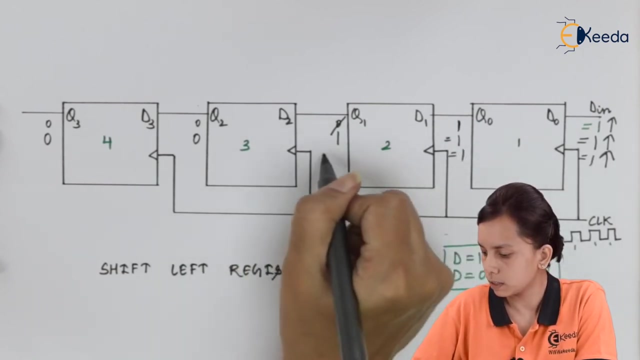 This q1 will change because d1 is 1.. This will be 1 and this is 0.. This is again 0.. No change. Again, I applied a clock pulse. This will be 1.. This is 1.. This is 1.. This is changed to 1.. 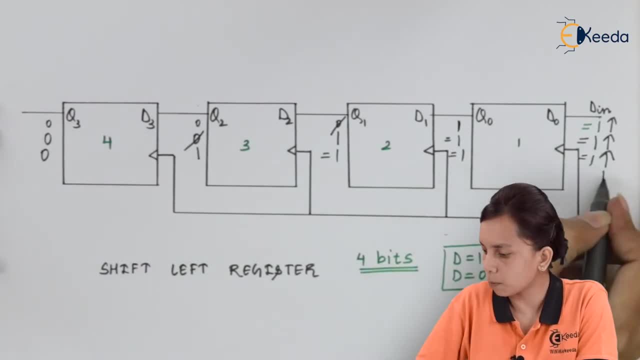 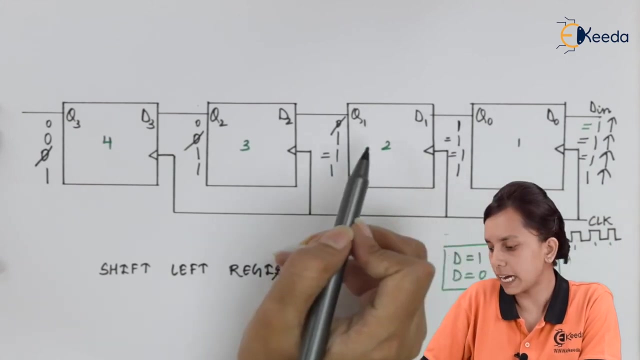 This is 0.. Again, I applied a clock pulse: 1, 1,, 1, 1, changed to 1.. So what we can say? that we are actually rotating our bit from this bit 1.. 1 was at this stage, then at this stage, this and this one, After applying 3 clock pulses. 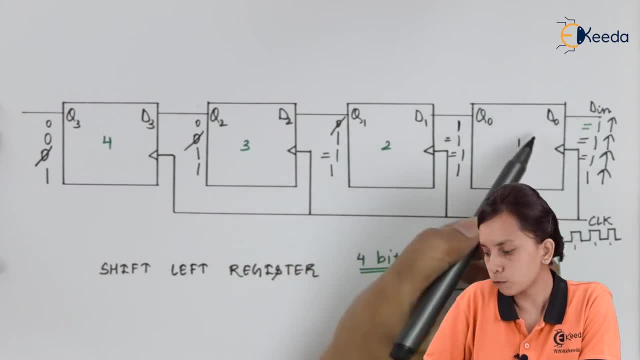 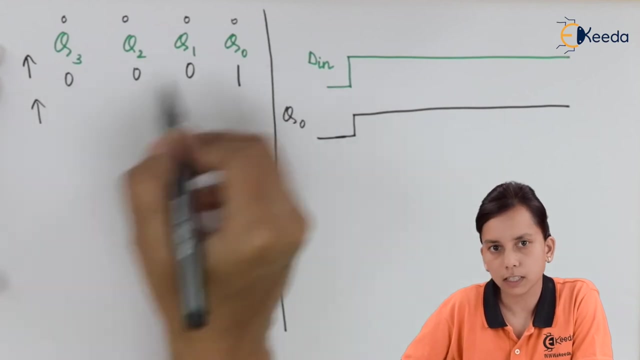 we are able to move this 1 from first, 1 to fourth, 1.. That's why I am saying that we are shifting our bit From first to second, second to third, third to fourth, What we are doing. Let us understand again, by the help of truth table, that at first clock pulse q0 is 1.. 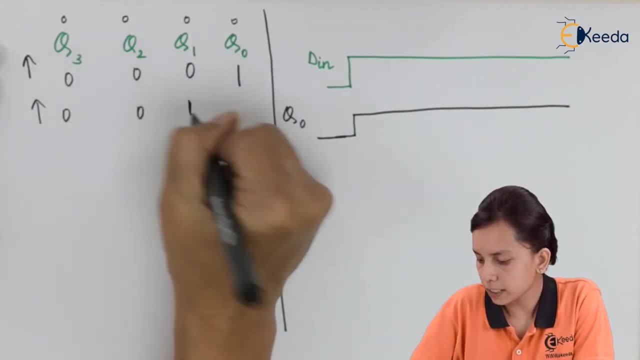 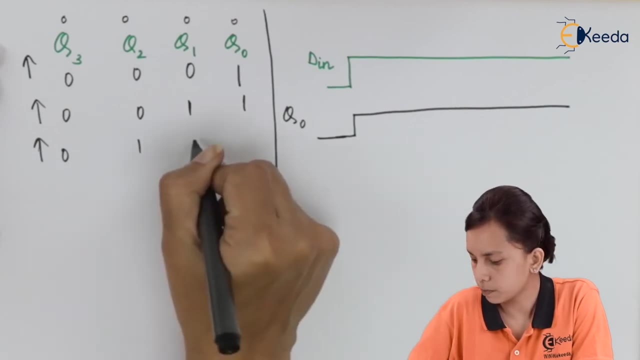 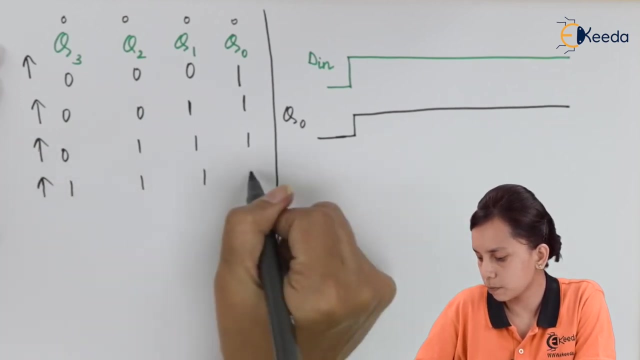 At second clock, pulse q1 is changed. At third clock, pulse q2 is changed and everything is same. Similarly, at the fourth clock, pulse q3 is changed. This is how I can say that my input was supposed to be at 1.. 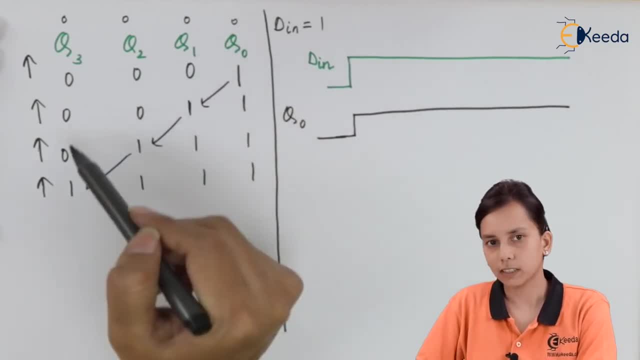 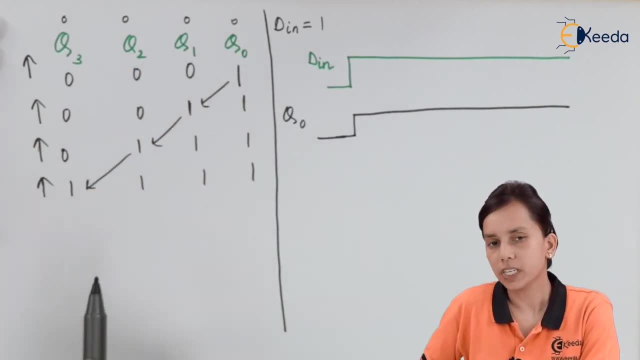 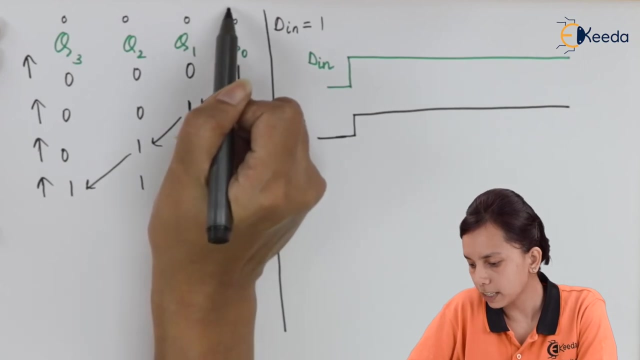 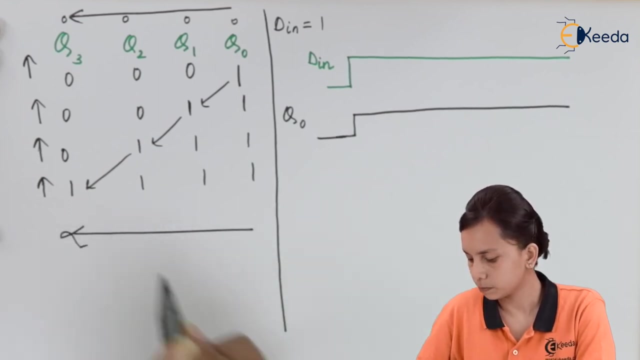 Now my beat is actually rotating. This is how I can say that when my beat is rotating, I can say that the particular register is rotating in nature, And when it is rotating such that it is going from, Let me write it down here- It is going from right to left. It is in the left direction. 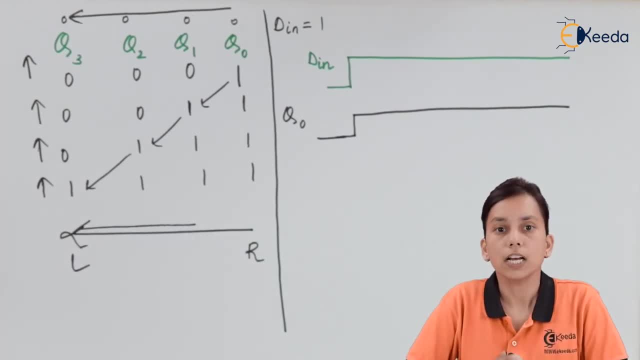 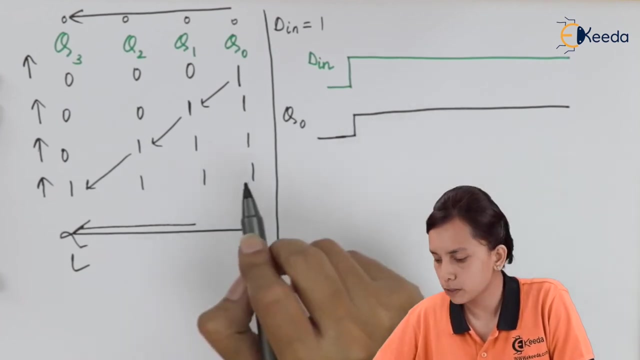 So we can say that this particular register is a shift left register because it is rotating its bit in a left direction. Let me draw the time diagram also. So this is for the Q0 that it will remains: 1. Let us say, this is our clock pulse. 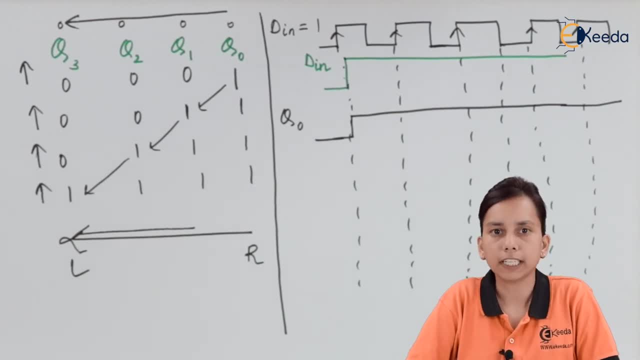 So in the timing diagram, what we are going to do is we are going to draw the time. What I will do that every time I will check the clock pulse and I will change the state in the respective order from Q0 to Q1, Q1 to Q and Q2 to Q3, and every time the previous. 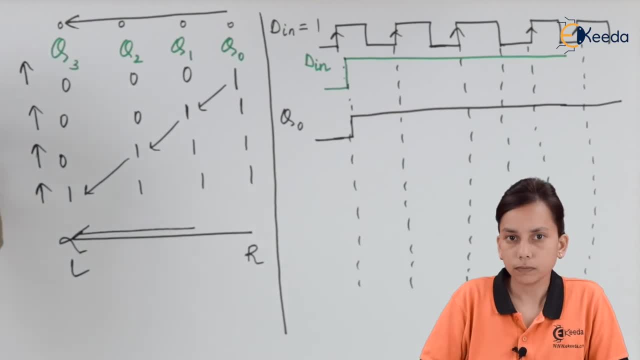 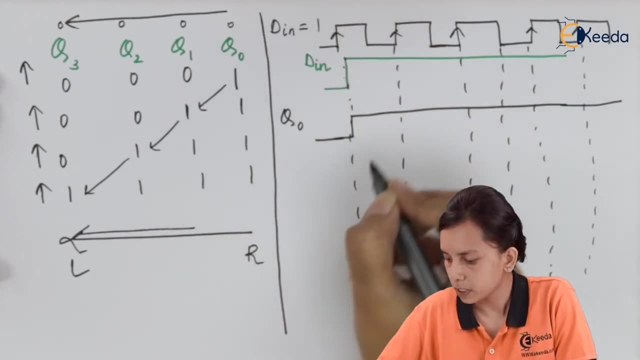 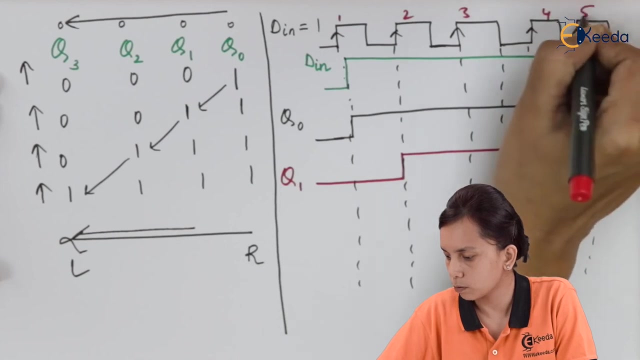 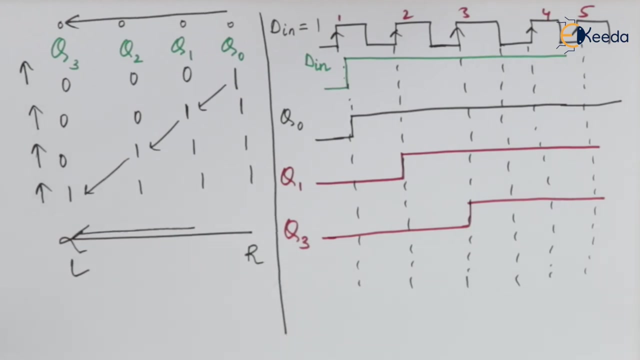 stages will be same. This is our Q0 at first clock pulse. Let us say now, at the second clock pulse, Q1 will change and it will be 1.. This is 1st, 2nd, 3rd, 4th, 5th and at the 3rd stage, Q3 will change. 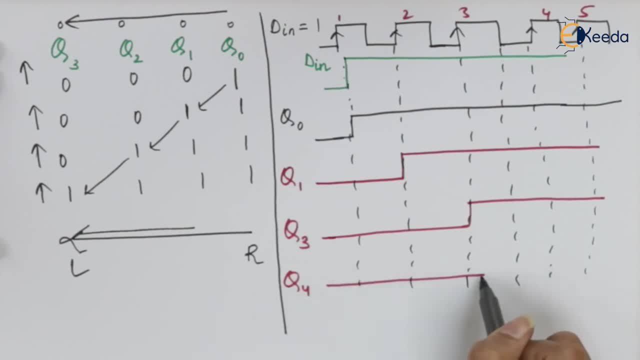 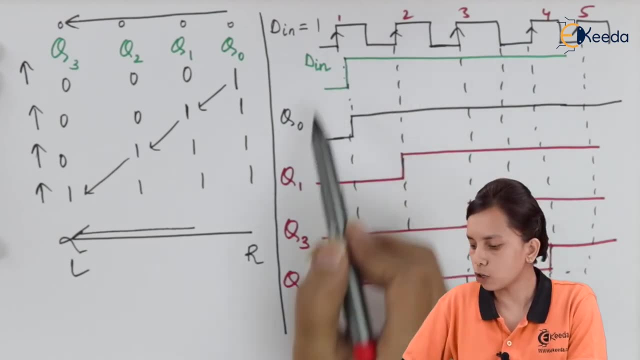 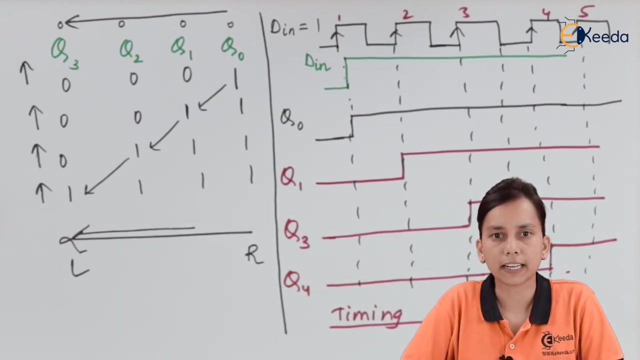 and at the 4th clock, pulse Q4 will change. So this is how we can draw the timing diagram for the particular type of shift register, And we can also store any type of address which is in a form of 4 bits. Suppose my purpose was to store 1, 1, 1, 1.. Then I can clearly instead. 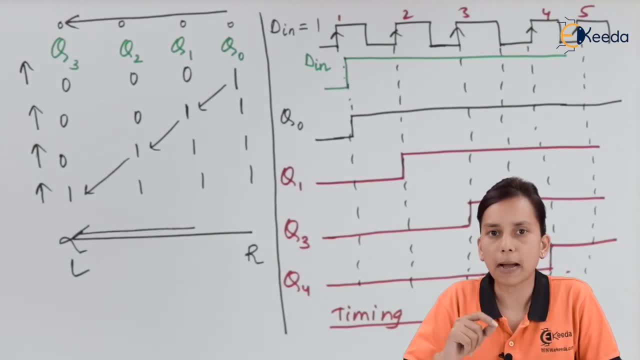 of rotating a bit, I can also put in my mind: yes, I want to design a circuit which can store 1, 1,, 1 and 1. by applying a 4 clock pulse I can store that particular pattern. So shift register can be used as a rotating register. and 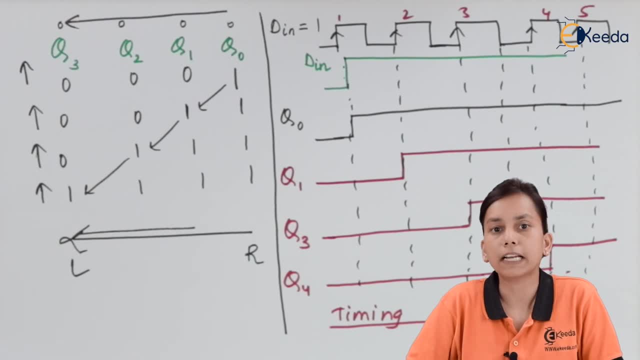 as well as a storing element When we are concerning about the 4 bit, because flip-flop is useful only for storing a bit, But, as all our devices, they are not the single bit 2 bit devices. They are up to GB. So for a GB we need a register. 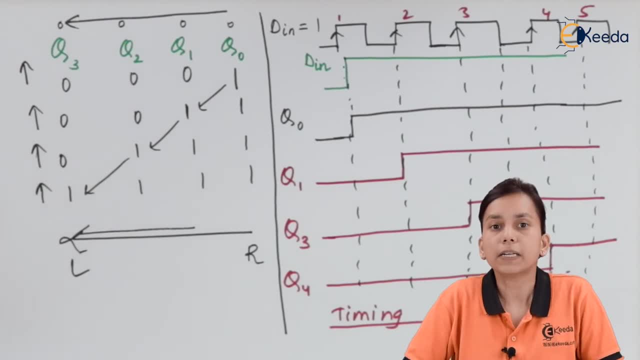 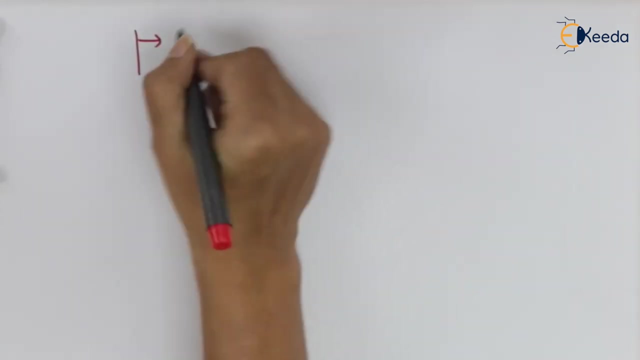 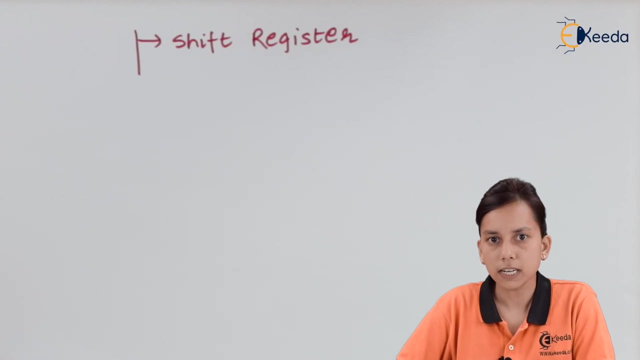 So register is not limited up to the rotating a bit. It can also be used in a storing more than 2 to 4 bits. So let us summarize our discussion. We understand the definition of the shift register. Then we understand the types of the shift register. 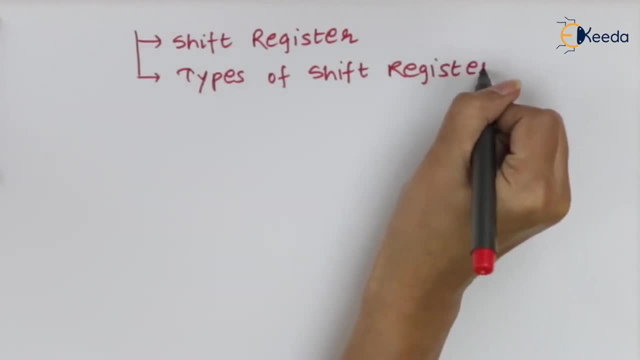 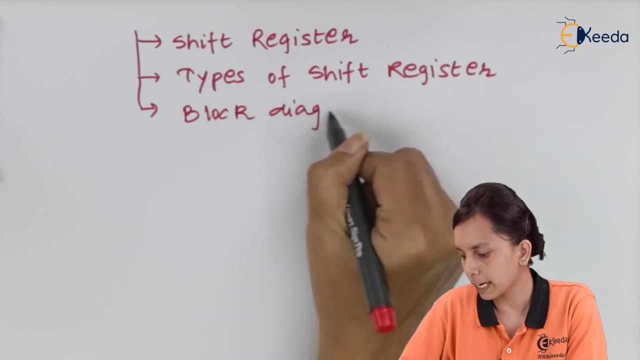 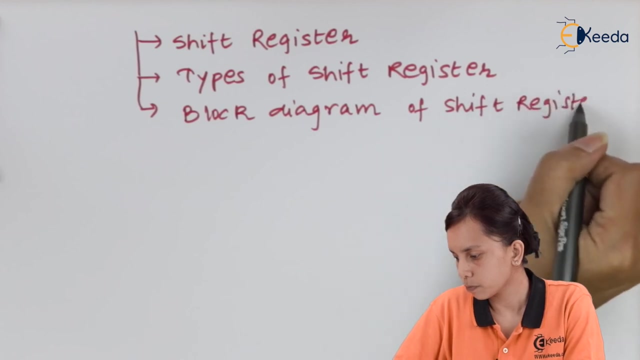 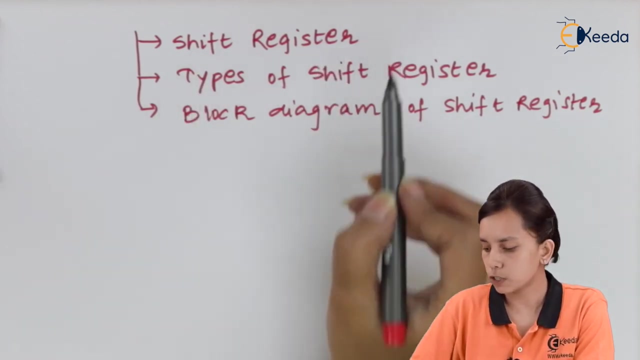 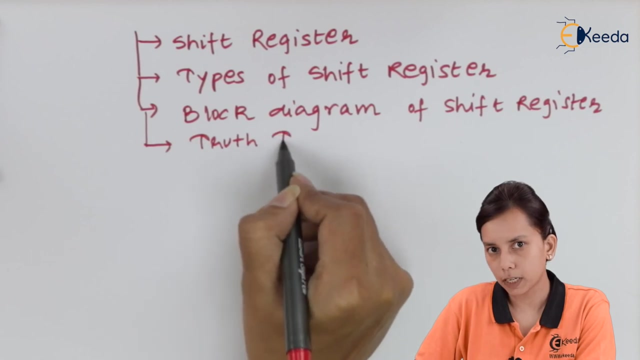 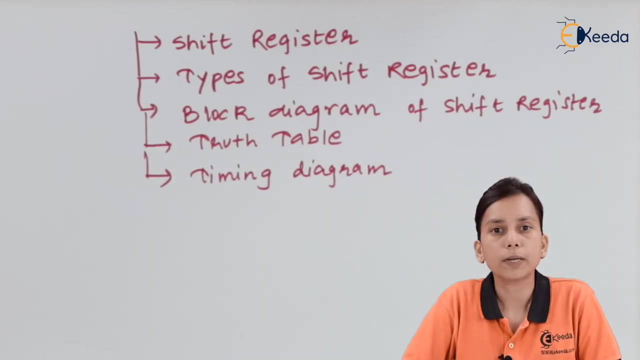 Then you can enter your method of: then we draw the block diagram of shift register in the exam. we will always follow this step, that first of all we will write down the definition, Then type, then block diagram through table. so it is very important that whenever we want to understand or we want to explain,